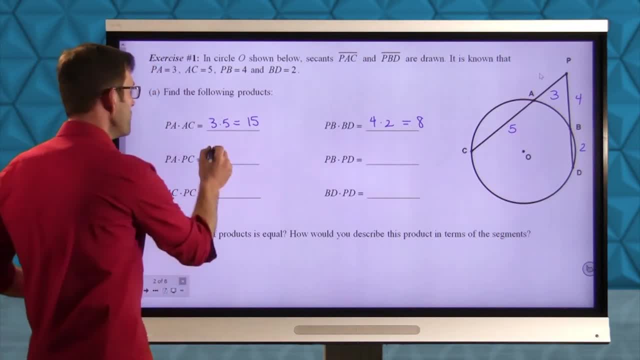 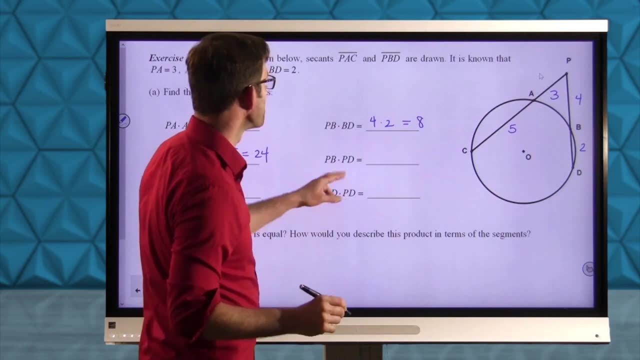 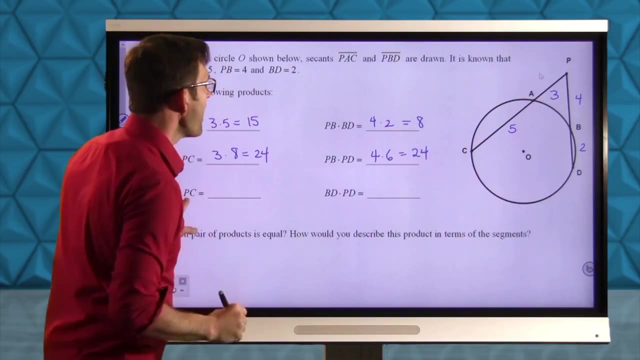 PC: PA times PC. Well, PA is three, PC, of course, is going to be eight, So then that's going to be 24.. PB times PD, That's going to be four times six, And that's going to be 24 as well. AC times PC. 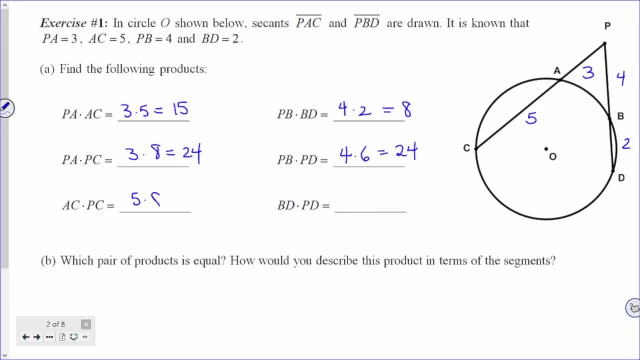 Well, AC is five Times eight, which is 40. And BD times PD, That's going to be two. Whoops, there's my two times six. Wow, this thing is just going crazy. Let's try that all the way over. Let's try two times six And 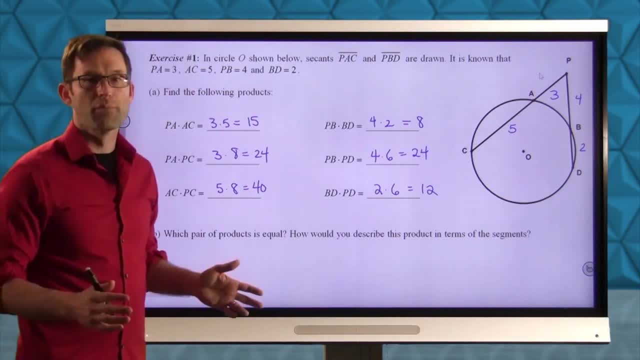 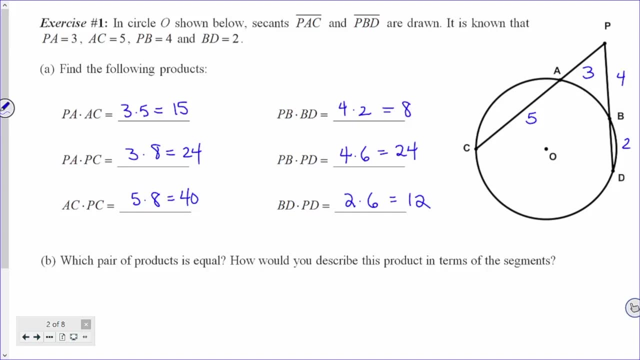 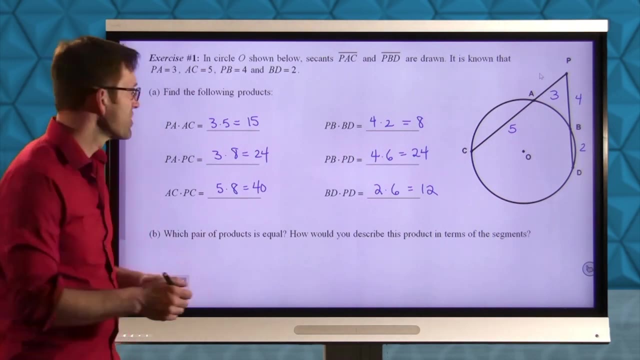 that's going to be 12.. All right now letter B, quite easy, asks us which pair of products is equal. How would you describe the products In terms of the segments? So there's one pair of these products That's obviously equal, And 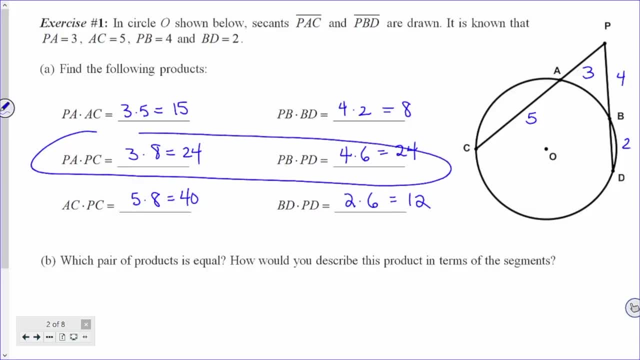 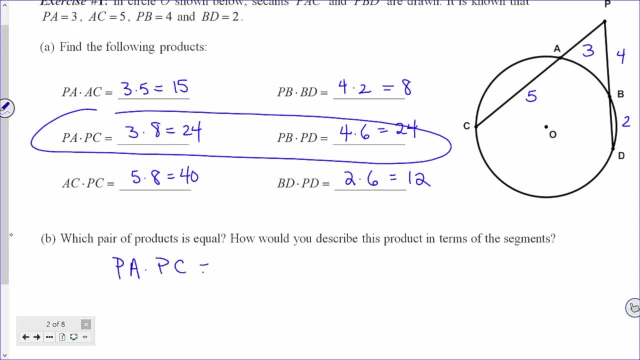 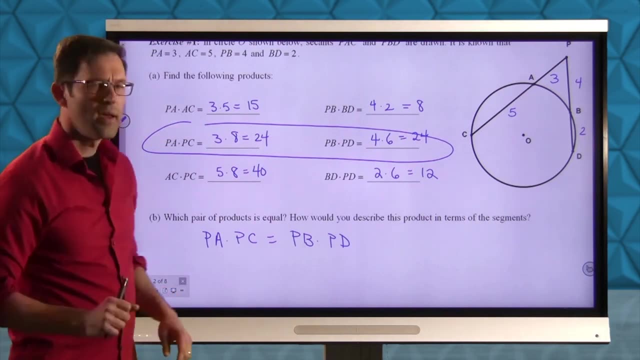 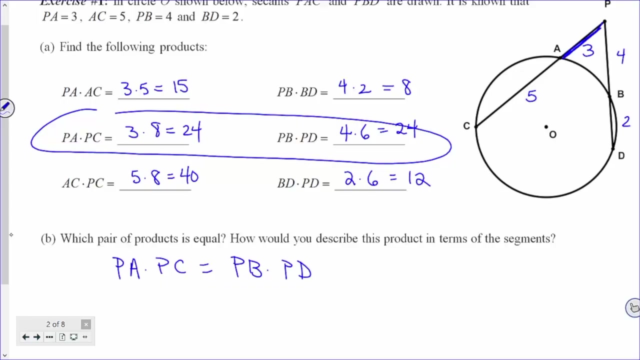 that's this one Right. In other words, trying to keep that up: PA times PC is equal to PB times PD. Okay, And how would we describe that? Let's, let's take a look: PA is this right, and maybe a different color, and PC is this length. all right, then, going back, PB is this length. 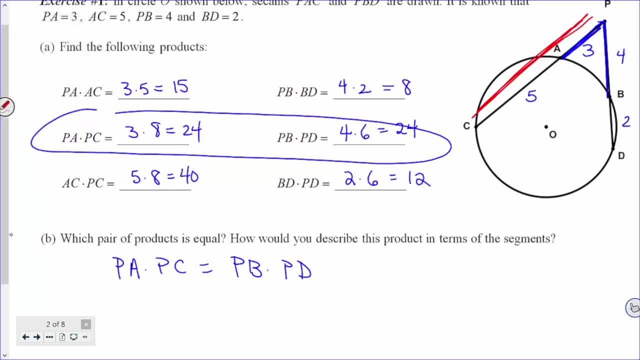 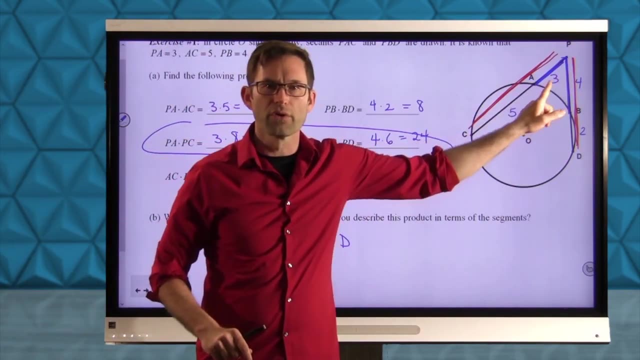 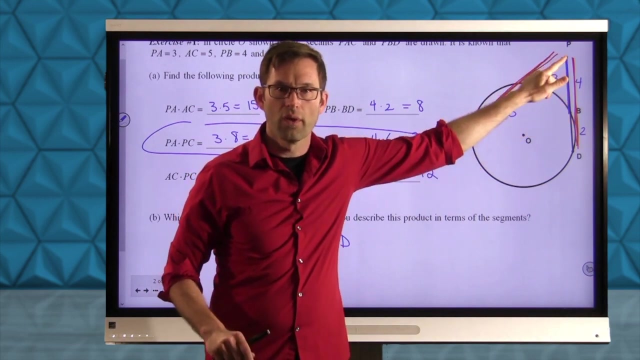 and PD is that length. so how could I describe that? well, we've got these two secants and it looks like when I take the portion that's exterior to the circle and I multiply it by the entire length, and then I take the portion that's exterior to the circle and I multiply, 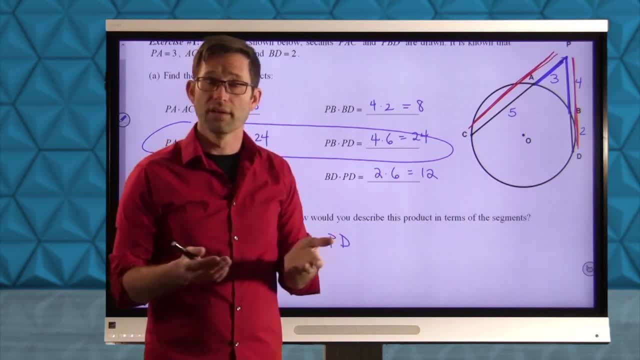 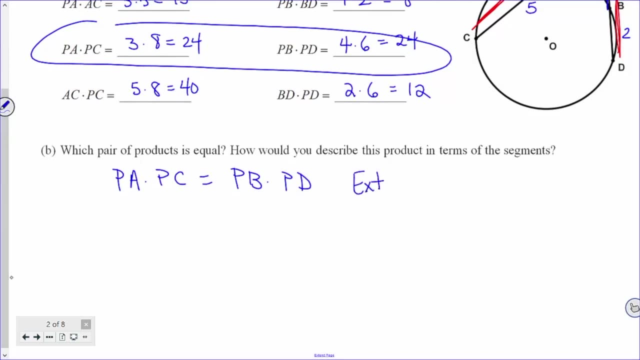 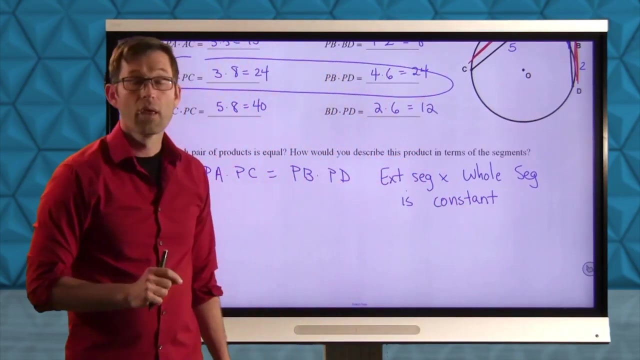 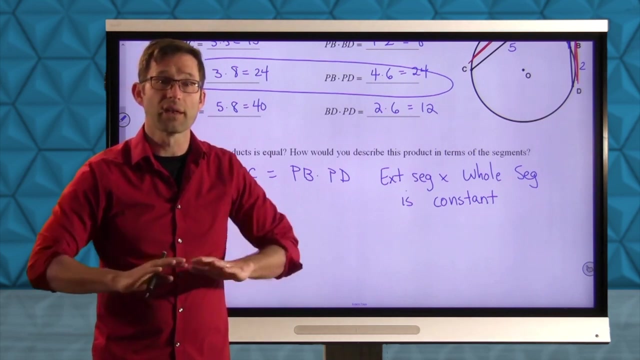 it by the entire length. it looks like that product is consistent or stays constant, so I think we would describe it as exterior segment times. whole segment is constant. so for every secant there's a portion of it that lies outside of the circle and then there's the entire length of that segment. we're assuming that the secant is 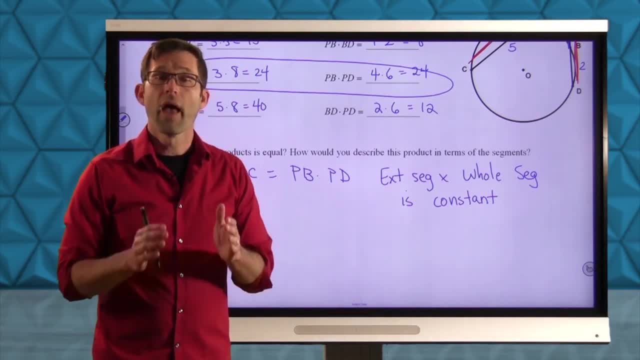 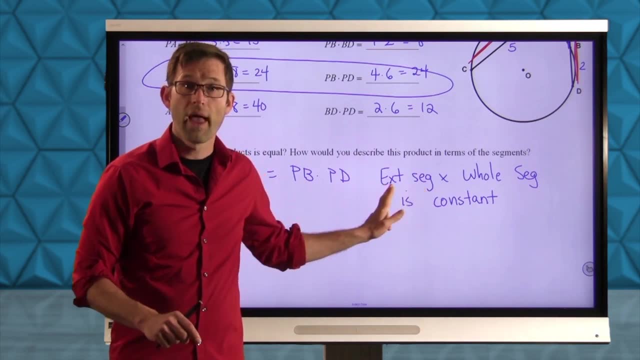 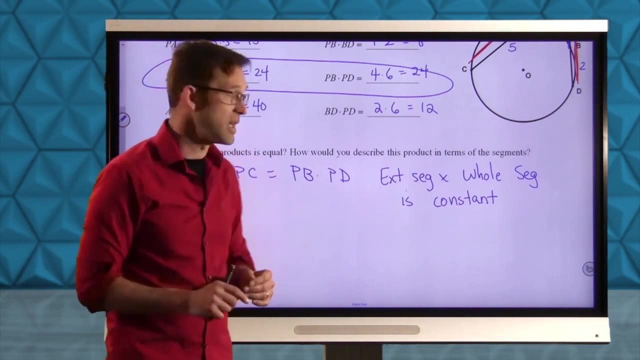 a segment, it's not continuing on forever, all right. and so it looks like- and this will be the case- that if we take the portion of the secant that's exterior to the circle and multiply it by the entire length, that product stays constant. all right, that product stays constant. let's kind of summarize that, if we can move, 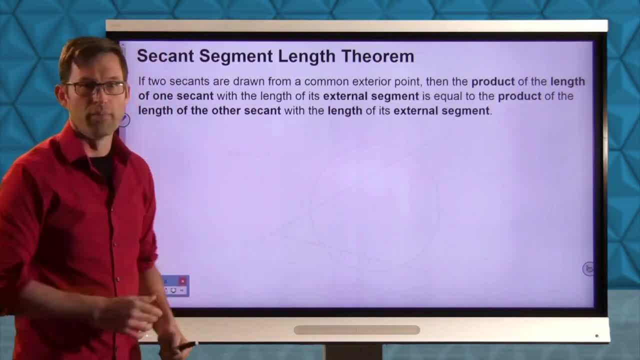 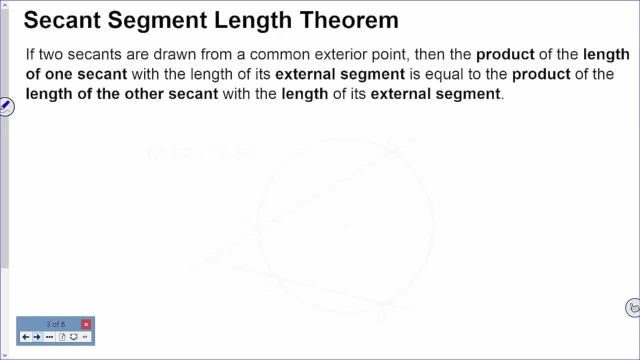 forward. there we go. secant segment length theorem. let's take a look: if two secants are drawn from a common exterior point, the product of the length of one segment with the length of its external segment is equal to the product of the length of the other secant with the length. 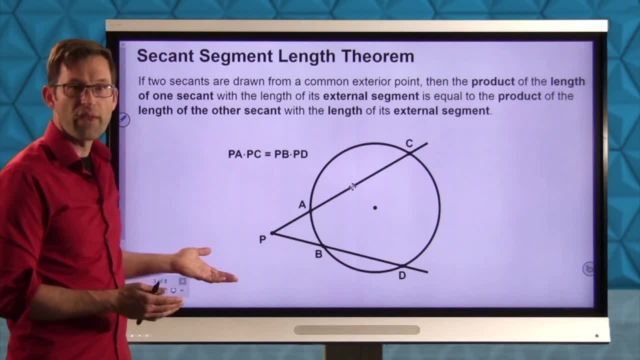 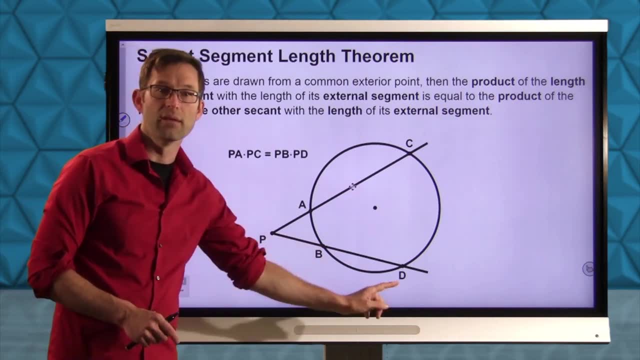 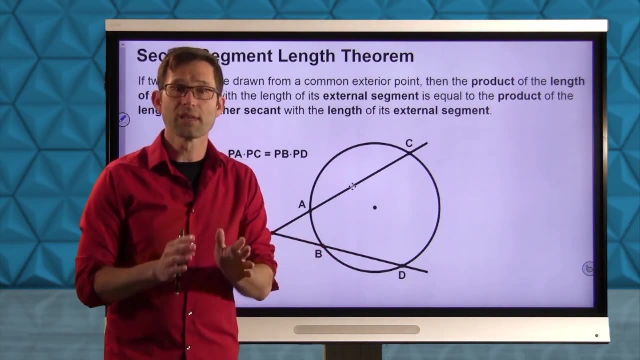 of its external segment. all right, so here we've got that picture. PA times PC is equal to PB times PD, and that's really the entire thing that we're going to be doing today, even when we get tangents involved. it'll be the same idea when we take the portion that's. 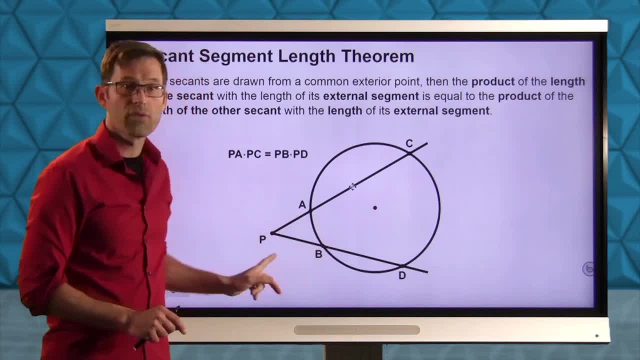 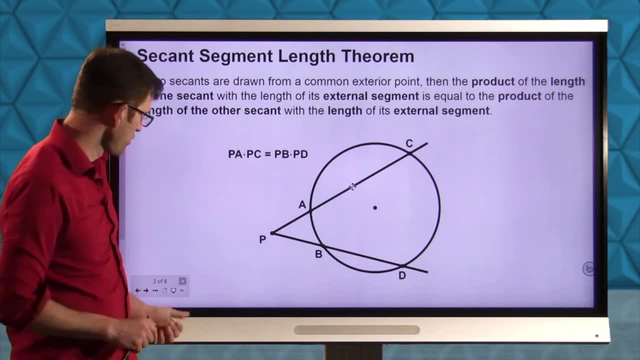 exterior to the circle and then we multiply it by the entire length. we'll get the portion exterior to the circle multiplied by the entire length, and we will eventually prove that. but first let's take a look at using it. it's an exceptionally easy theorem to use. let's take 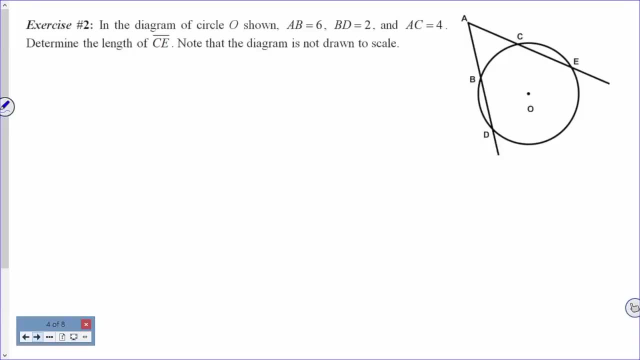 a look at exercise two. in the diagram of circle O shown, AB is equal to six. all right, let's label that BD is equal to two, AC is equal to four and we want to know the length of CE. now, of course, the incorrect way of using this theorem is to say, okay, six times two equals four times X, and then 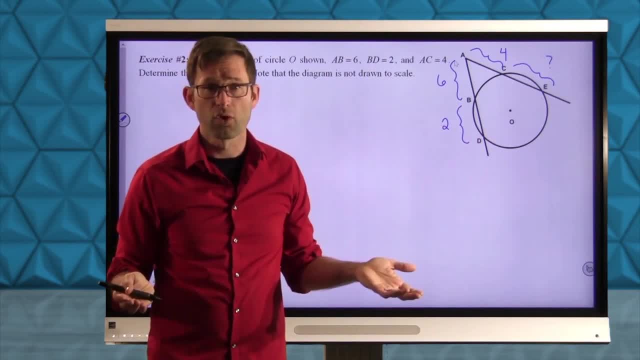 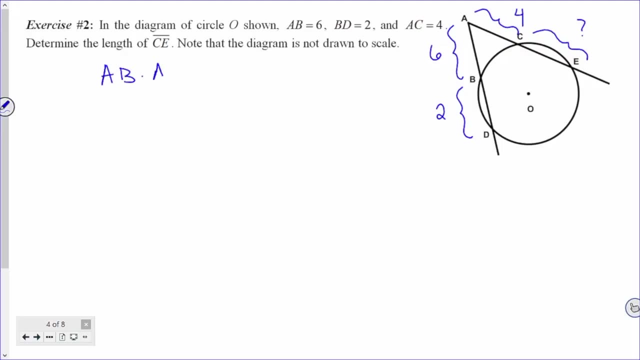 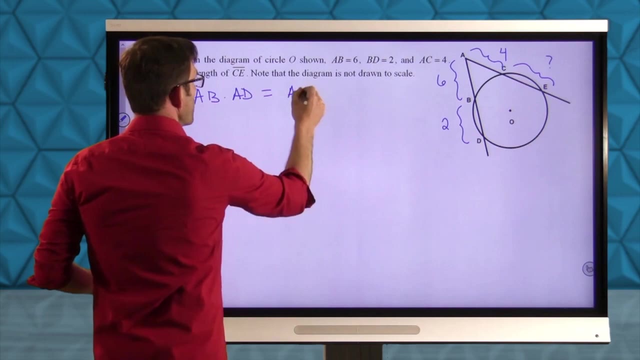 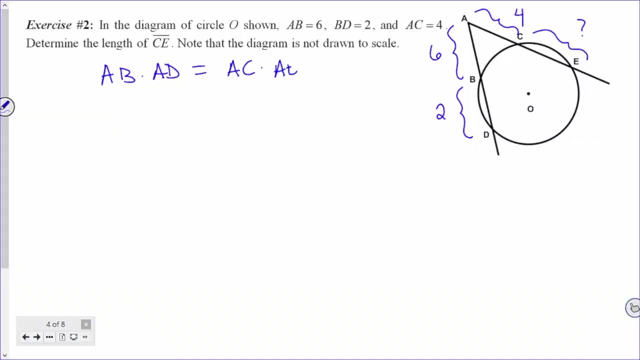 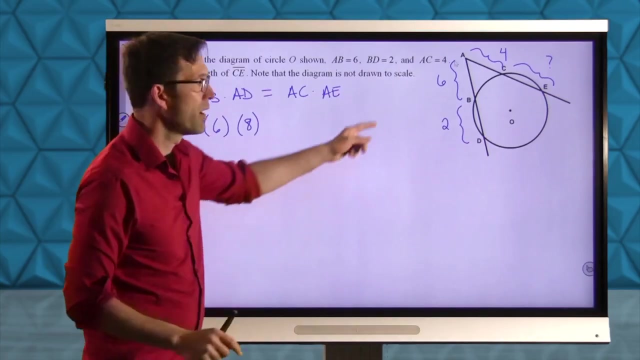 solving for X, that would give me X equals three, and it would be incorrect. okay, what the theorem says is: it says that AB times AD, right? AB times AD is equal to AC, AC times AE. now just kind of filling the blanks. well, AB is equal to six. AD, though, is equal to eight, right I? 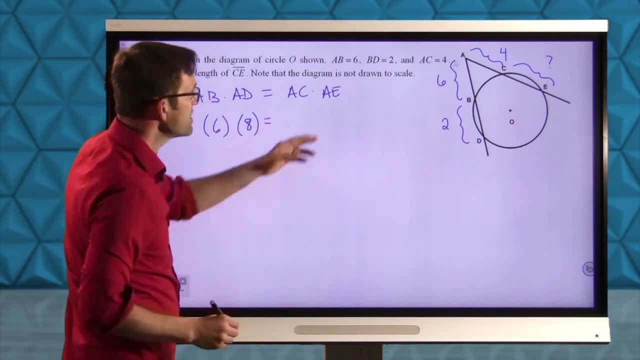 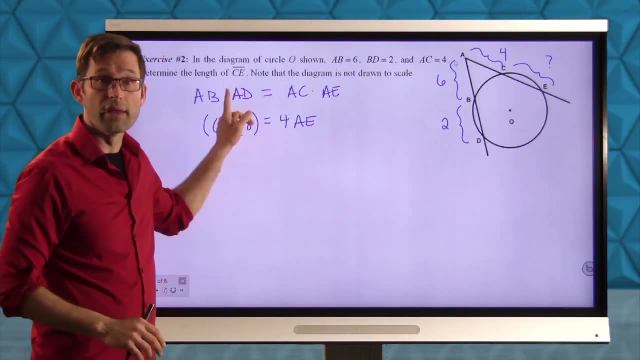 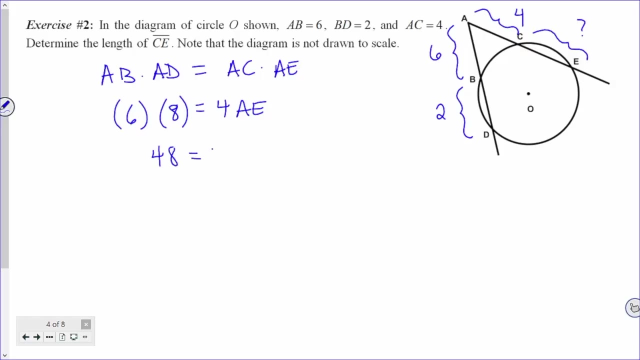 have a. six plus two. AC is equal to four, and this will now let me solve for AE. granted, I'm not actually looking for AE. I really want the length of CE, but I need AE to find it. this is simple enough. six times eight is 48, four times AE. divide both sides by four. 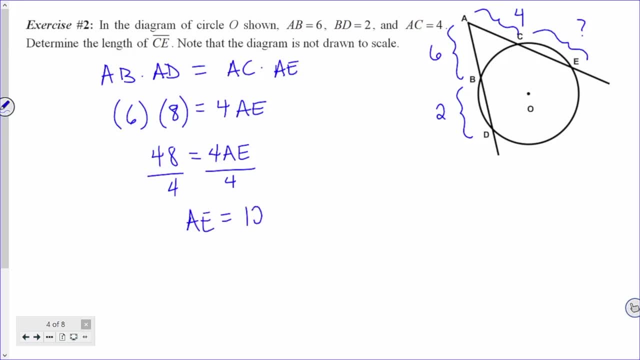 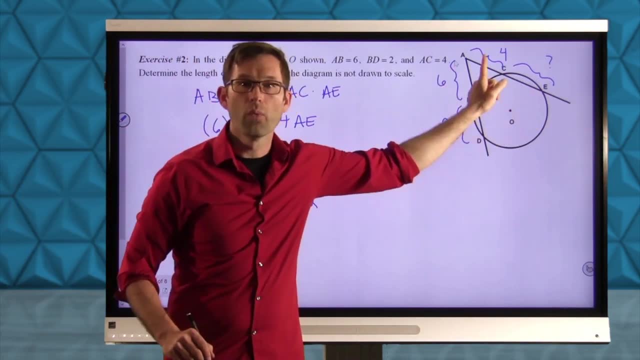 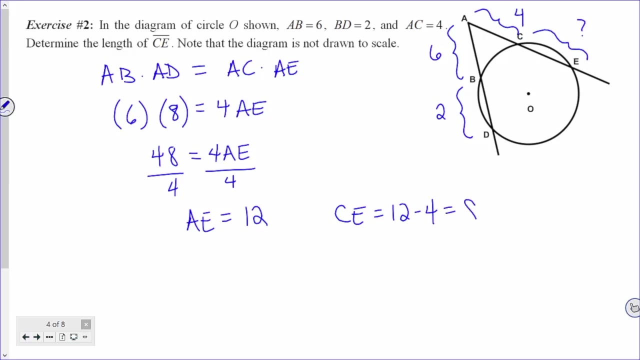 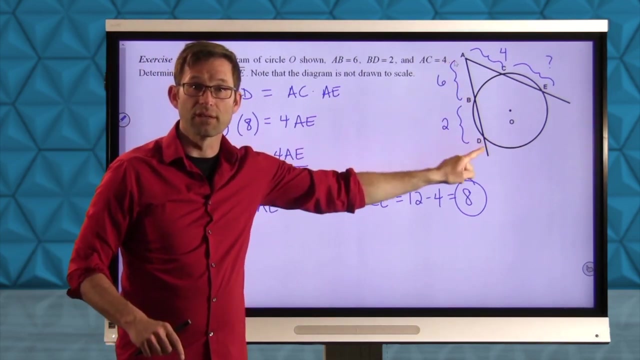 right and what we find is that AE is equal to 12.. and because we now know that the length of this entire segment, AE, is 12, we can just subtract off the four and we find that CE must be 12 minus four. CE's got to be eight. that's it. exterior segment times the entire length equals exterior segment. 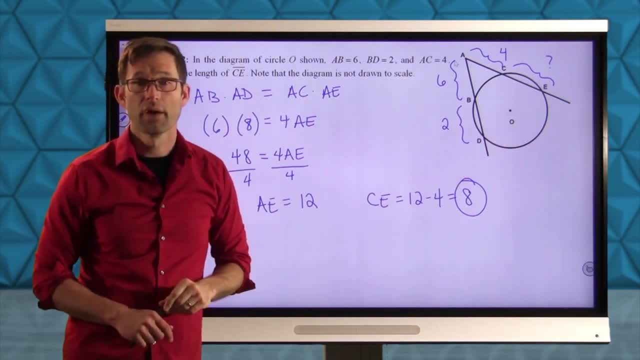 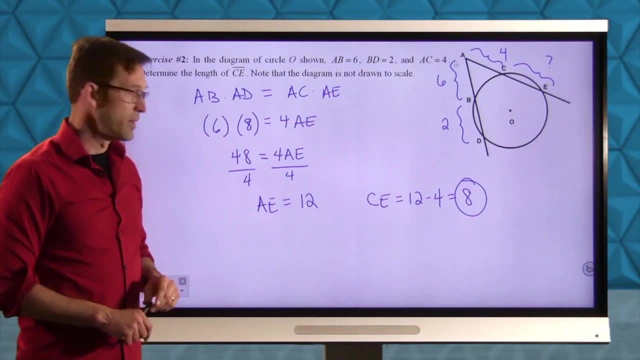 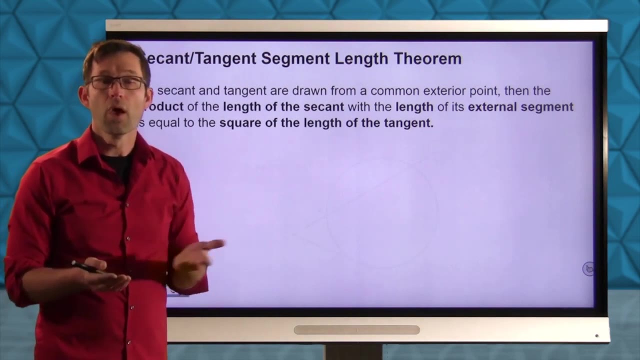 times the entire length. it's the whole deal. all right, let me step out of the way so you can write something down and then we'll move on. all right, let's do it. okay now, what happens if we have a secant and a tangent? we won't even really. 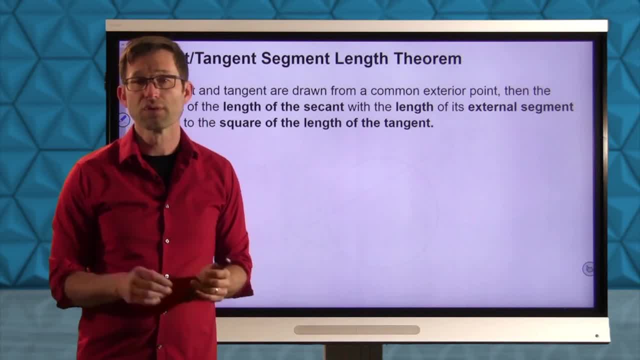 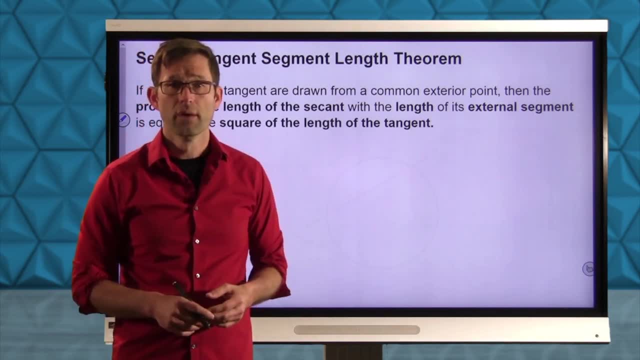 talk about two tangents because, quite frankly, when you have two tangents, something that we learned before was that the length of the two tangents have to be equal. so there's no real fancy theorem for that, other than the length of the two tangents have to be equal. but let's take 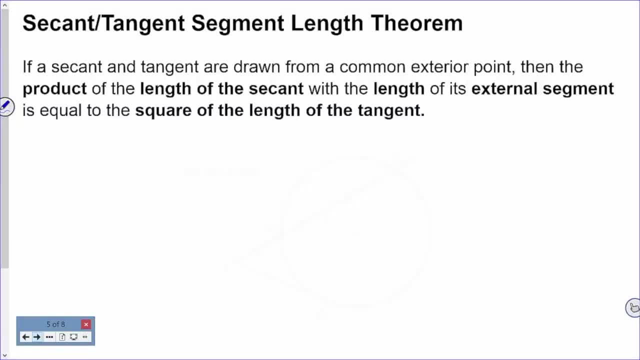 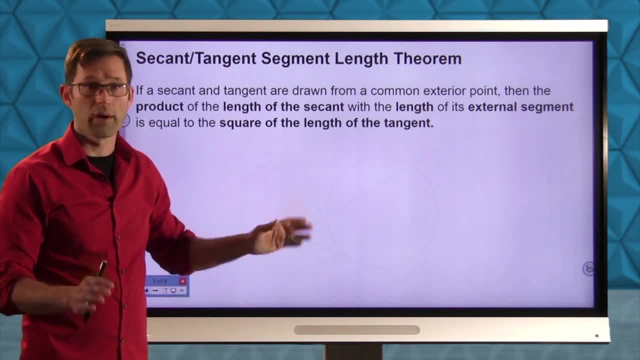 a guess. if a secant and a tangent are drawn from a common exterior point, then the product of the length of the secant with the length of its external segment. so that's the same thing as we had before. all right, we're taking a look at the total segment times. the external segment is: 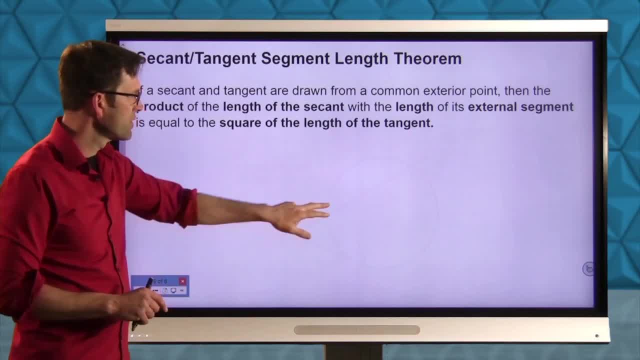 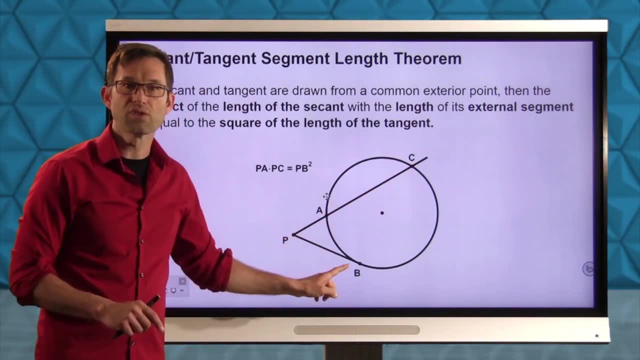 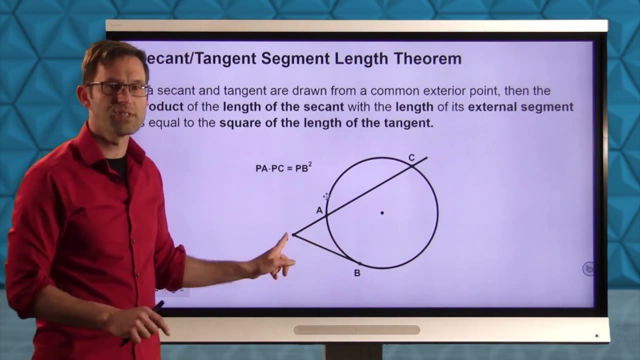 equal to the square of the length of the tangent. wow, another theorem to memorize. right, so we've got PA times. PC is equal to PB squared. now that almost seems like it's a different theorem than the word, than the one we had before, But keep in mind the one that we had before said. 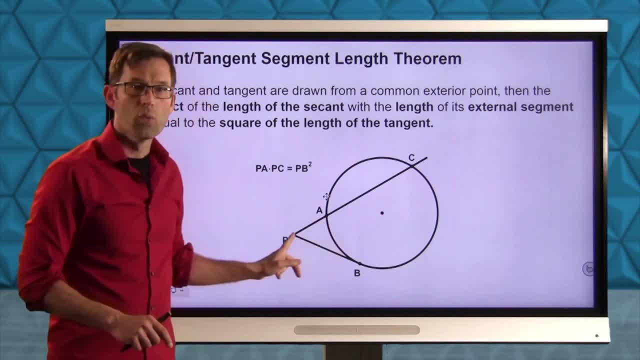 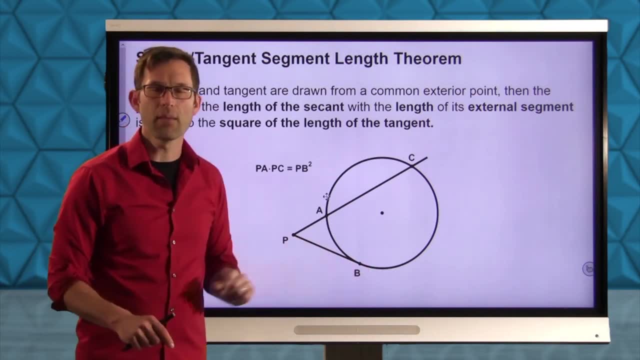 if we take the external segment and multiply it by the whole thing, we'll get the external segment multiplied by the whole thing. But the external segment and the whole thing are the same for a tangent And that's why we just get the pb squared. 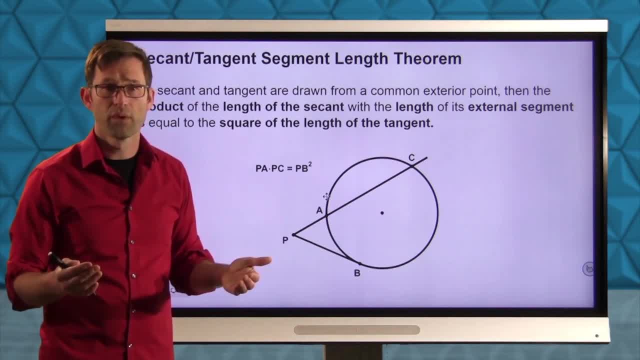 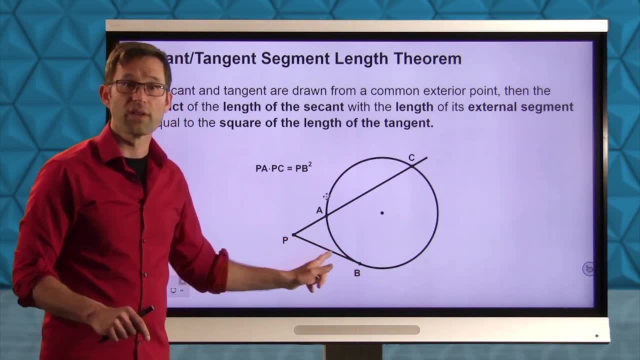 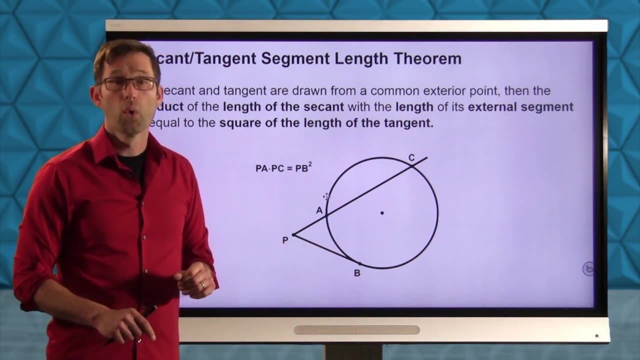 So it's absolutely, absolutely the same theorem. It just happens that with a tangent, its entire length is exterior to the circle. So when we take the exterior length and we multiply it by the whole length, we just get the length of the tangent squared. 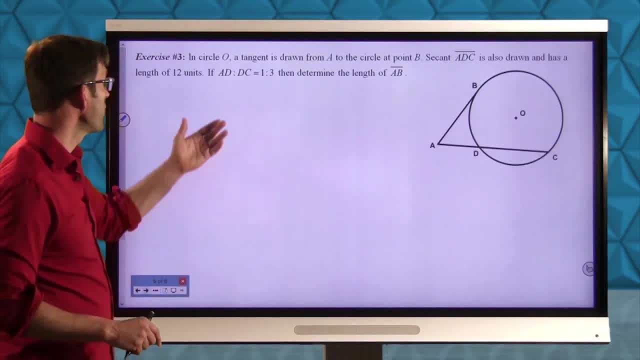 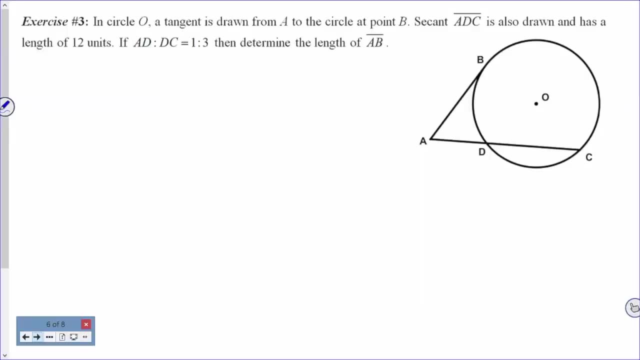 All right, let's use it. It's an easy enough theorem to use, just like below. Let's take a look. Or before exercise number three: In circle O, a tangent is drawn from A to the circle. at point B, Secant ADC is also drawn and has a length of 12 units. 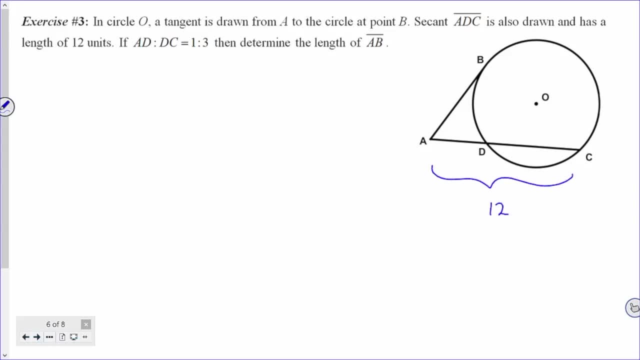 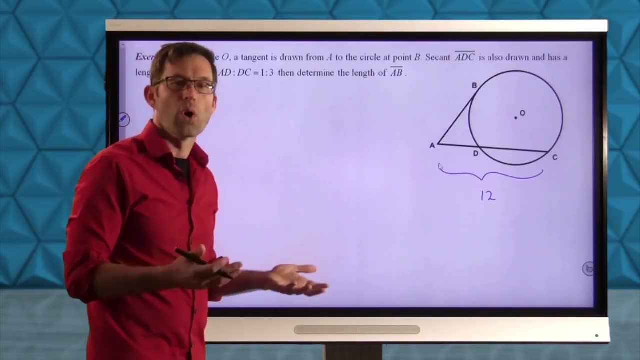 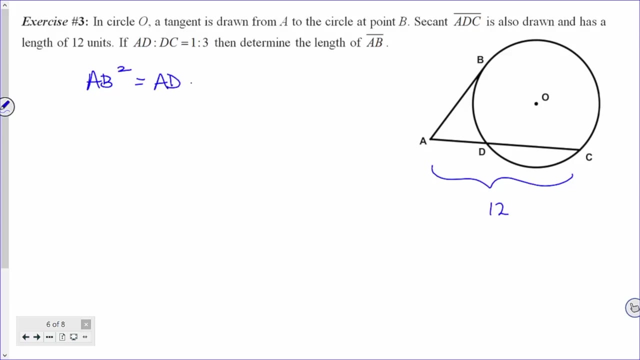 So we know that this is 12 units. If AD to DC is equal to 12 units, then ADC is 1 to 3, determine the length of AB. All right, so the theorem says that if I take AB and I square it, I'll get AD times AC. 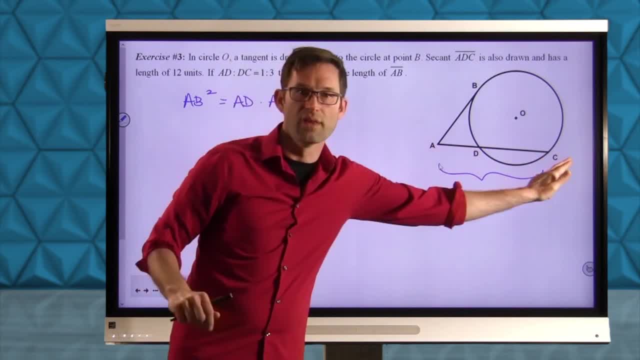 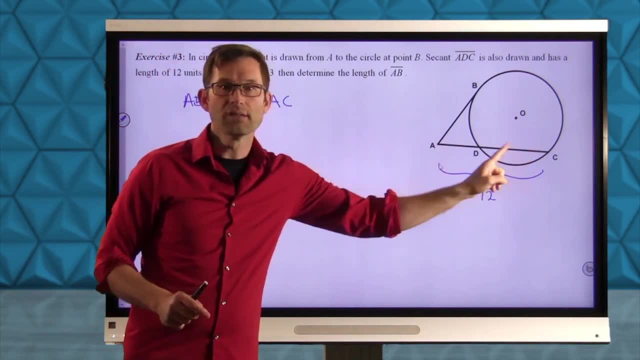 So this times this is equal to this. times this AB squared is AD times AC. The problem is, although I do know what AC is, it's 12, I don't yet know what AD is, And that's where I've got to do that. 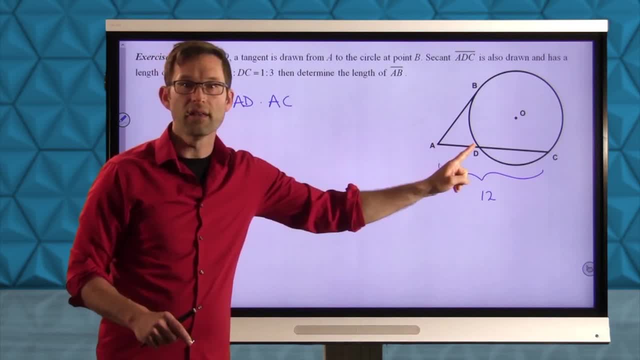 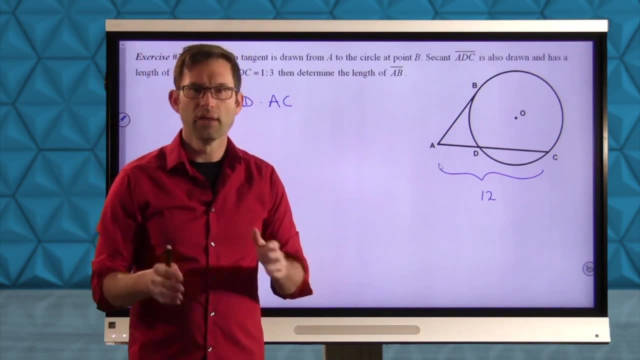 piece with the ratios, right. I know that the ratio of AD to DC is 1 to 3.. Now many of you can probably just kind of go: oh, all right, then AD must be blank, OK, but if you don't, then we go with one of these again. 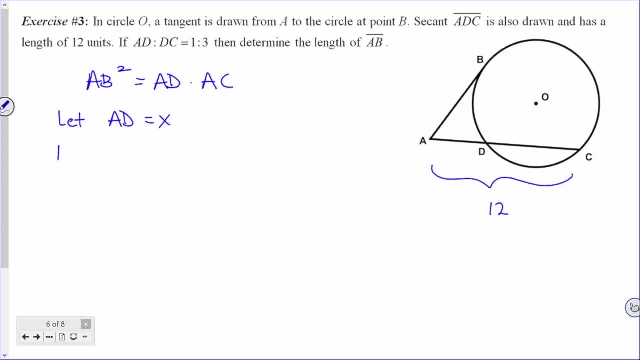 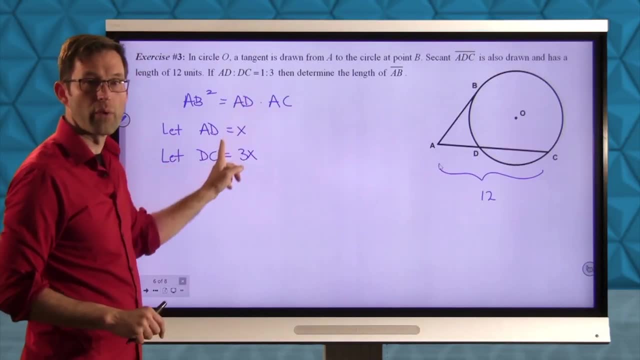 We'll let AD be equal to x, We'll let DC equal 3x, right, That maintains that 1 to 3 ratio, 1x to 3x. Then I can use sort of the same thing. I can use sort of the same thing. 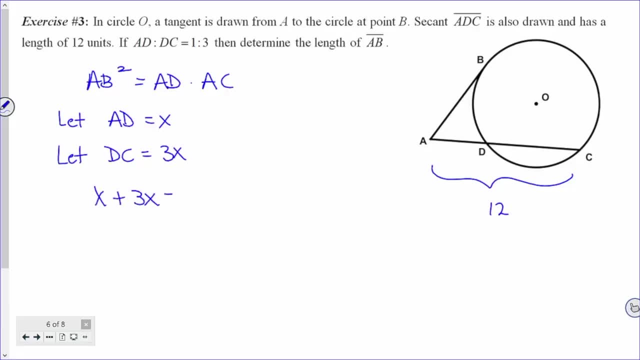 I can use sort of the same thing. I can use sort of this whole as the sum of its parts. to say, x plus 3x has to be 12, right, When I add the two together, I've got to get those 12 units. 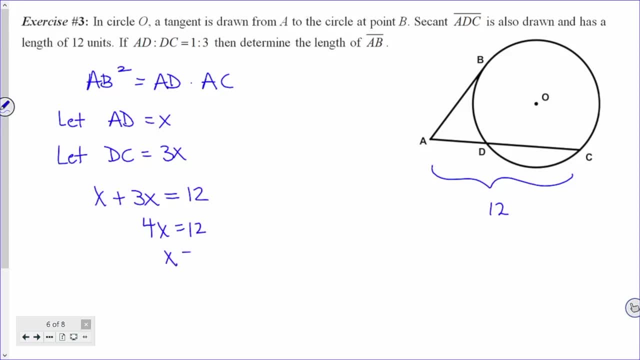 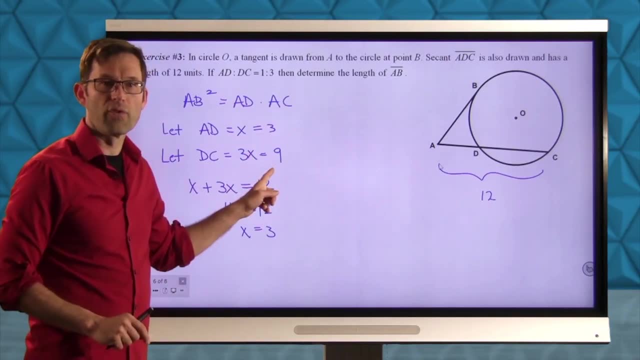 So 4x must be 12 and x must be 3,, which means AD is 3 and DC is 9.. I don't really need the 9, though, and I want to be careful not to use it. I really just needed that 3.. 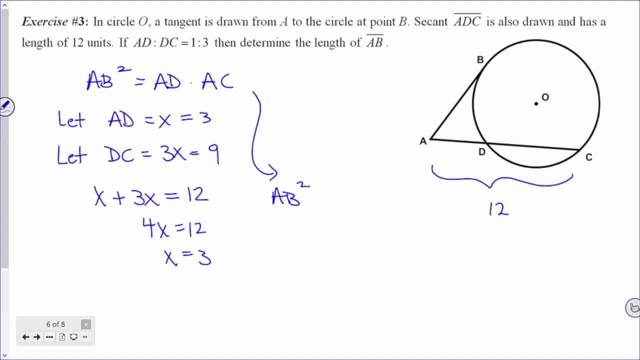 So now I can say that AB squared is equal to AD, which is 3, times AC 12, AB squared is equal to 36, take the square root of both sides and AB is 6,. all right, Not too bad right. 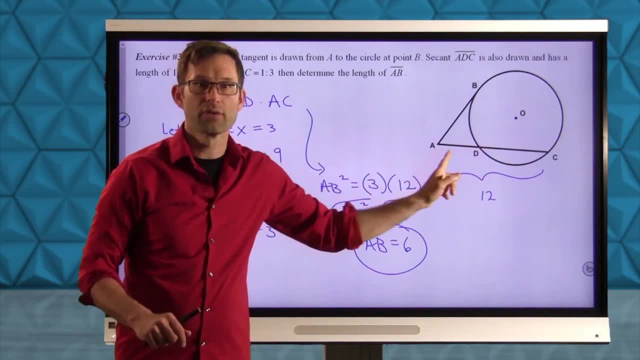 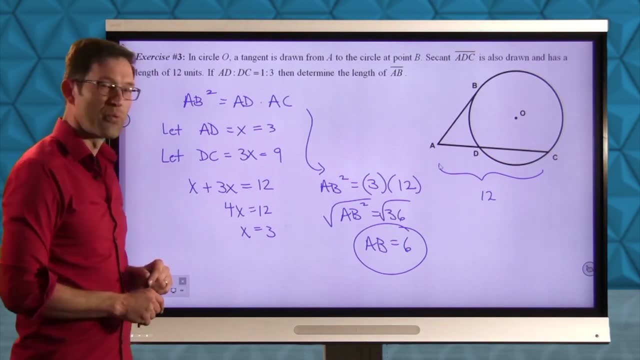 The exterior times. the whole is equal to the exterior times the whole. That's the theorem. Let me step back, write down anything you need to, then we'll go on and we'll prove this thing. All right? All right, let's do it. 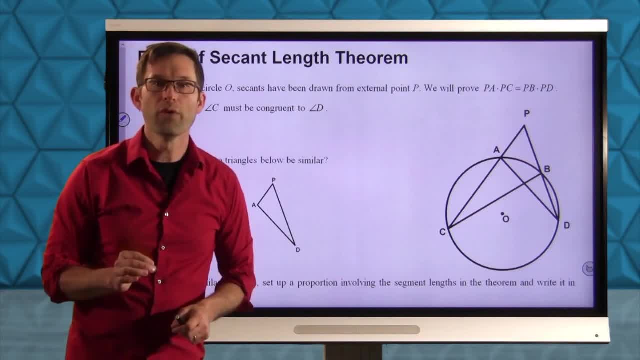 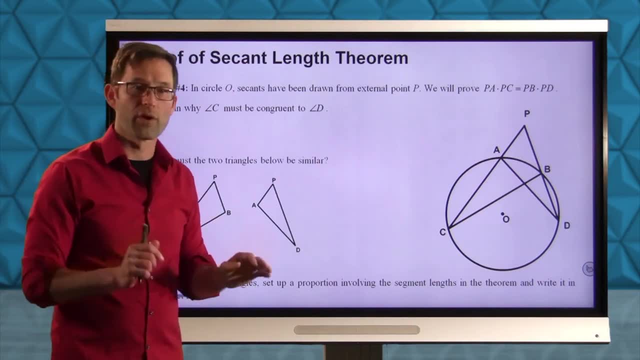 So the last exercise: we're going to prove the secant length theorem. So we're not going to do the tangent length That's going to show up on the homework, We're going to prove the secant length theorem. And again, let me give you a little bit of a setup. 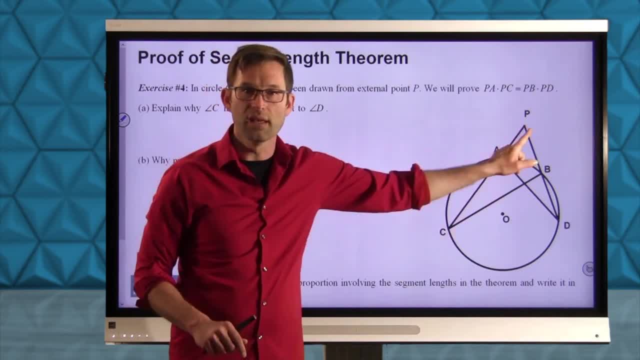 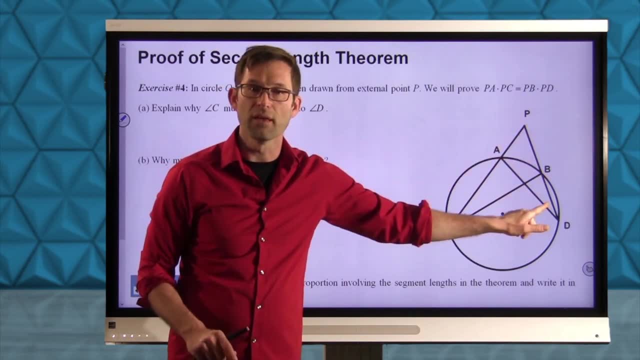 What we've got right now is we've got these two secants drawn: PAC and PBC. OK, And again, I want to prove that PA times PC is equal to PB times PD. In order to do this, I had to draw these extra lengths in, OK. 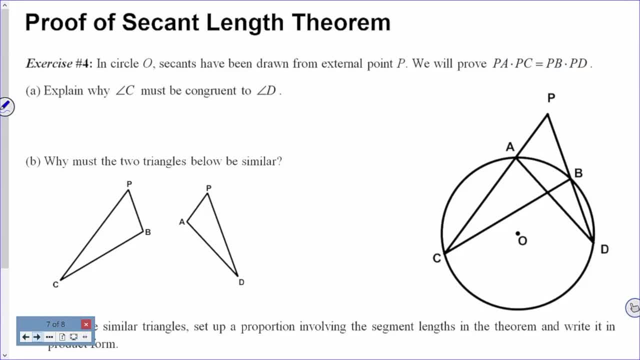 And let's kind of take a look. OK, exercise number four: In circle O, secants have been drawn from external point P. We will prove PA times. PC equals PB times. PD Letter A. Explain why angle C must be congruent to angle D. 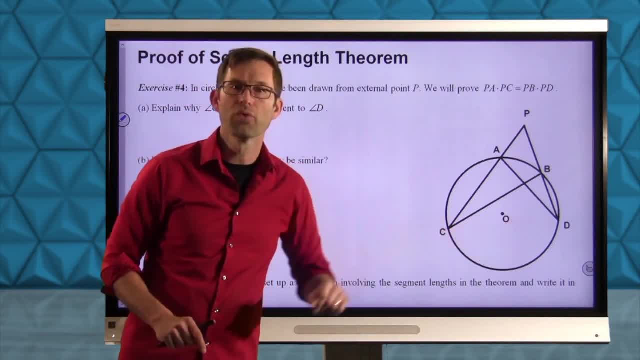 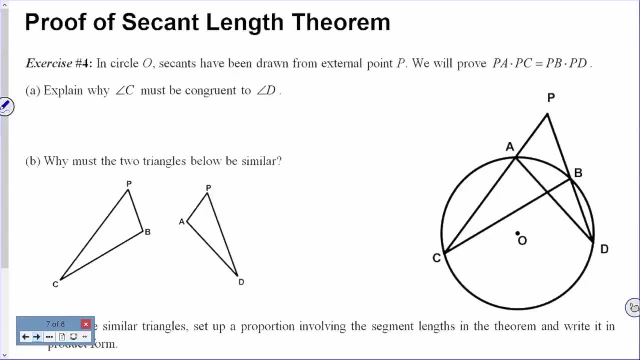 Why does this angle, angle C, have to be congruent to angle D? Pause the video now and see if you can answer this question. All right, well, it's because They are both inscribed angles. They are both inscribed angles that intercept the same arc. 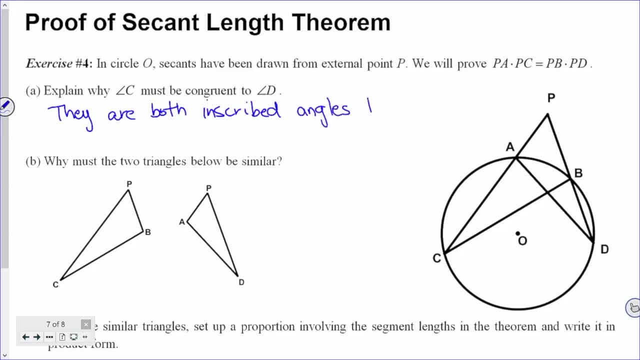 Specifically arc AB, But whatever right. So they both are intercepting the angle, okay. That's why angle P is congruent to angle D. So let's do this again. We have a angle like this. We have angle P, angle B. 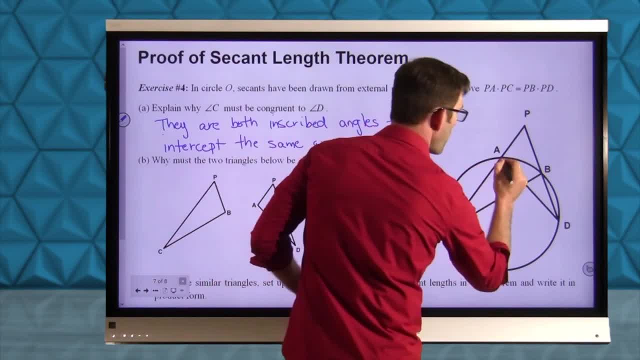 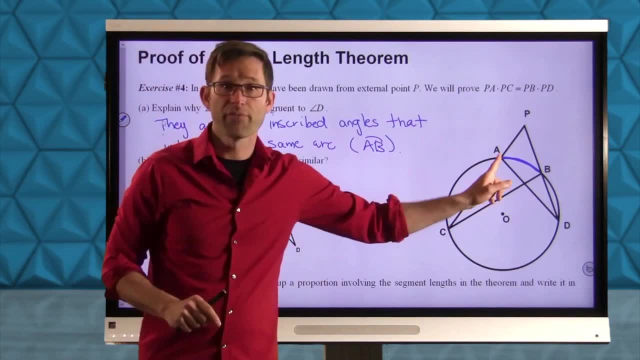 We have angle A and angle B, We have angle B, I have angle B or intersecting arc AB And again, since they have to be half the measure of arc AB, that means they both must be the same measurement. So if arc AB is 60 degrees, 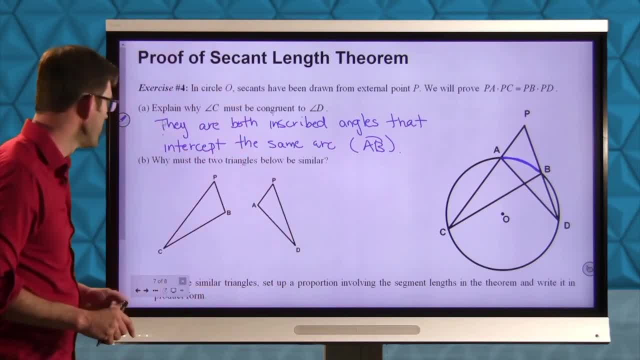 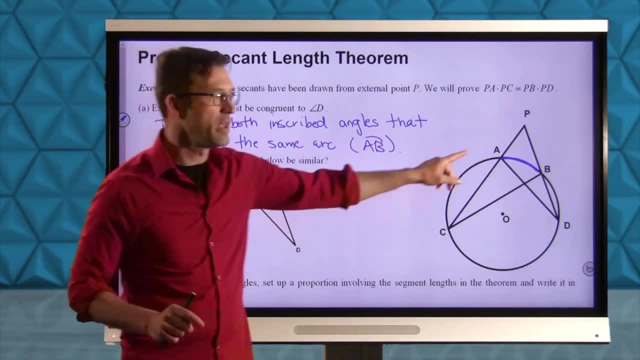 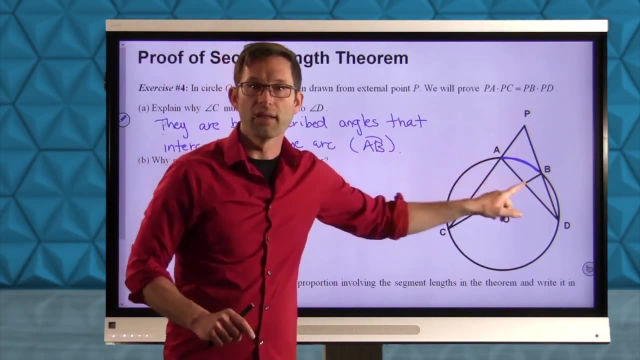 C and D are both 30 degrees Letter B: Why must these two triangles be similar? Now again, keep in mind that what I've done is I've taken triangle PCB right here and triangle PAD and I've just kinda put them here. 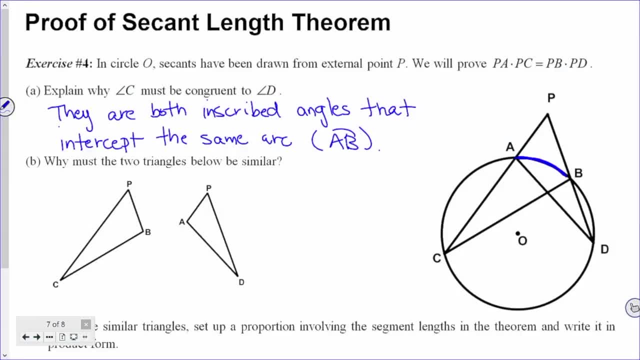 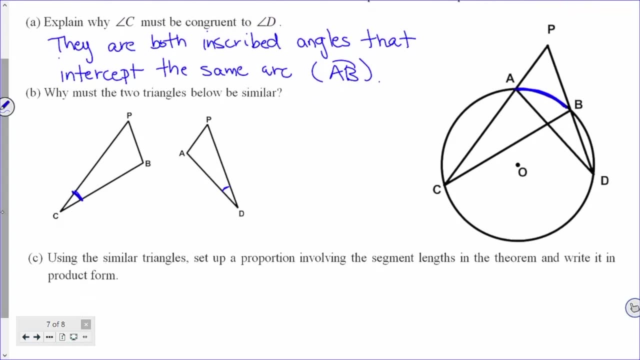 Why do those two triangles have to be similar? Well, let's take a look. Number one: we just proved, or explained, why angle C and angle D must be congruent to each other, But one of the beautiful things here is that they also 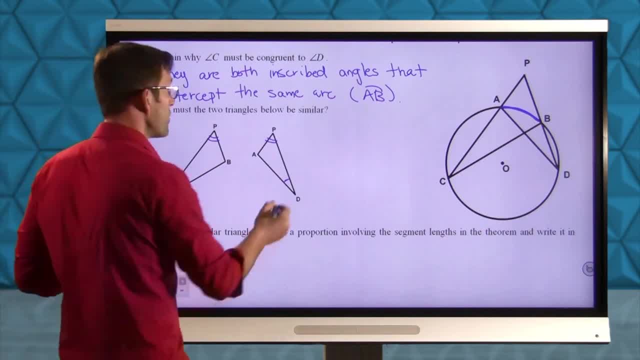 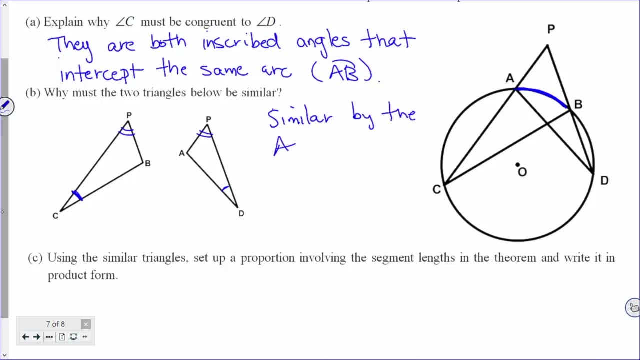 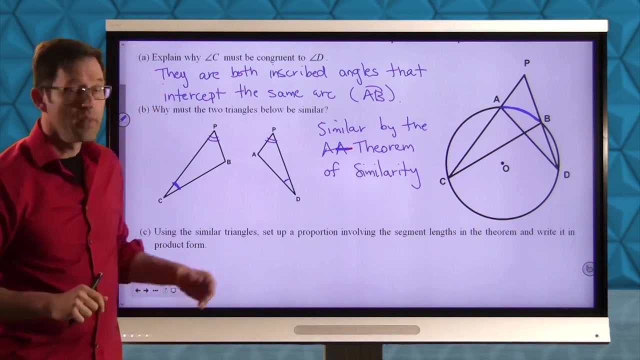 share an angle. They share angle P, And so they're similar by the angle-angle theorem of similarity. Hey, red pen. It's been a little while since we've seen red pen There. we'll just cross it out. Okay, They're similar by the angle-angle theorem of similarity. 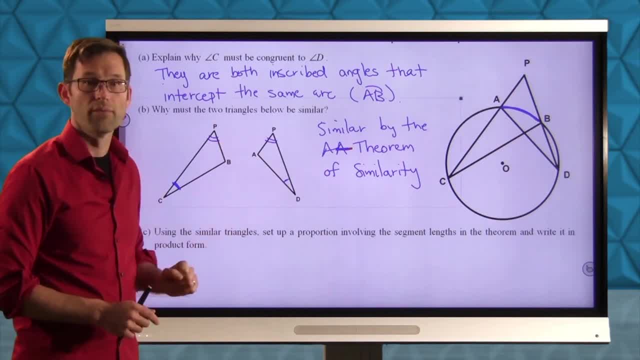 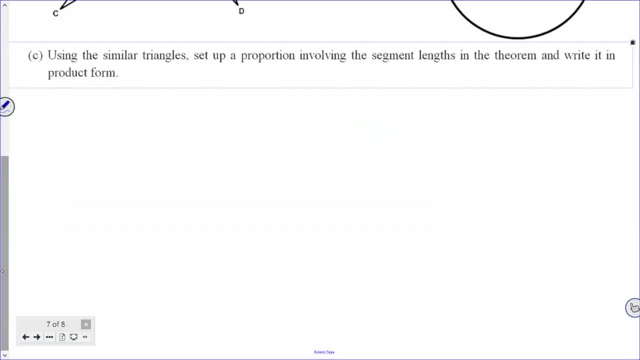 There they are: Angle equal to an angle, angle equal to an angle. Great, Now let's finish the proof. This is going to be simple, Right? It says: using a proportion, or using similar triangles, set up a proportion involving the segment lengths. 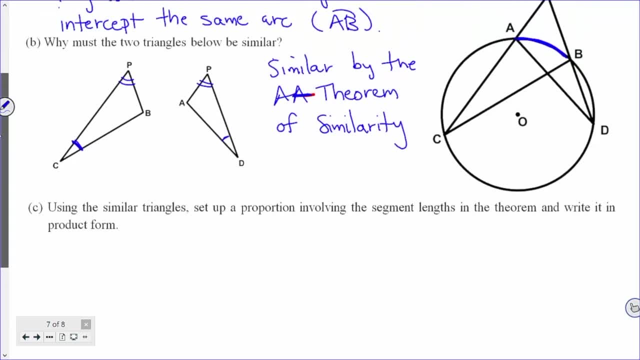 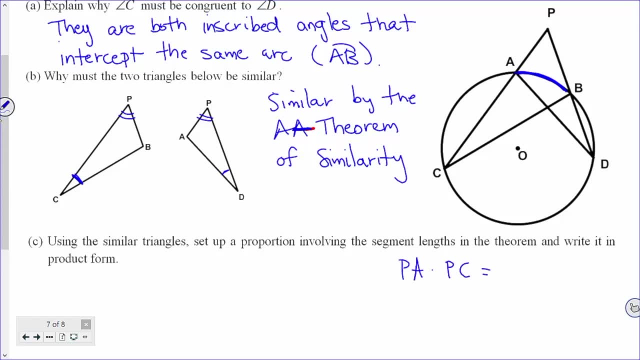 in the theorem and write it in product form, And remember what I'm looking to do. Right, Let's write down what we really want. We want to get the fact that PA times PC is equal to PB times PD. Right, That's, at the end of the day, what I want. 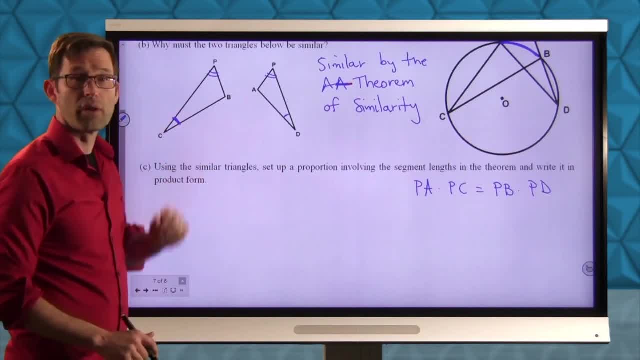 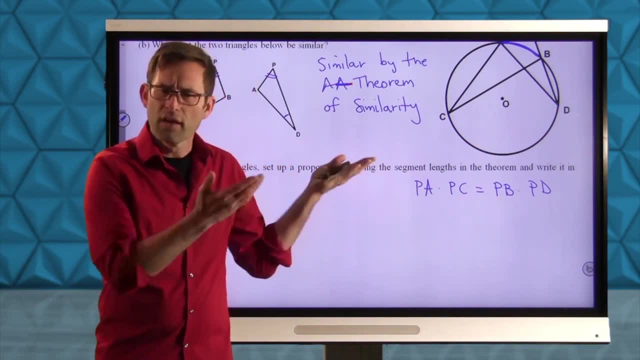 I just want to be able to bring it up here. And now it's all about the similarity of these two triangles. Keep in mind, right, those similarity proofs we did where the final line was to prove some product. Well, that's really in geometry, to set us up for proving something. 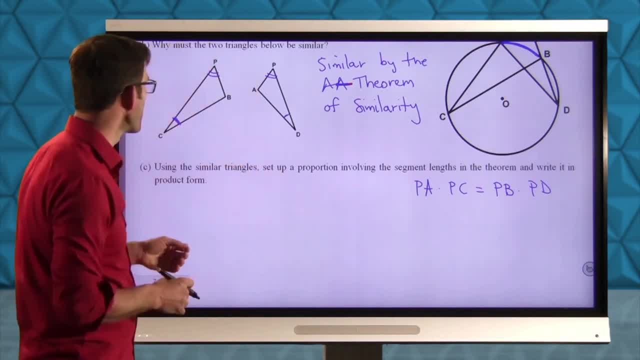 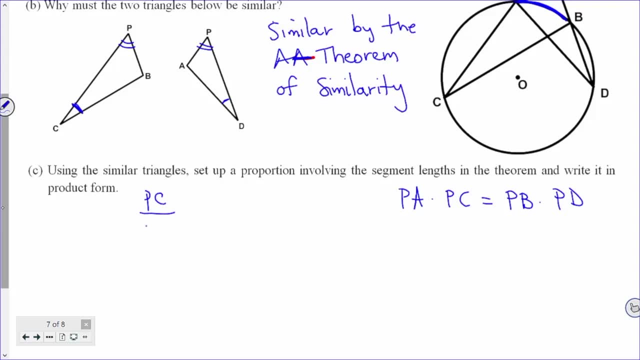 like this. So let's like, let's do that similarity piece right. What we know is that we know that if I do PC divided by PD, all right. if I do PC divided by PD, I'm going to get- I would have to get- PB divided by. 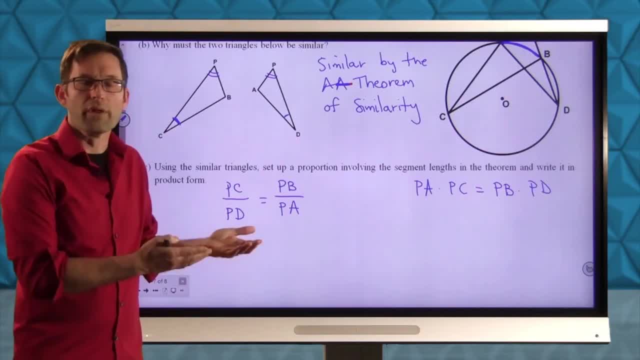 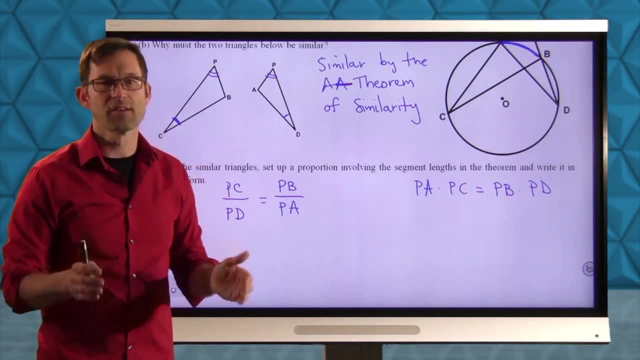 PA. All right, And if we were doing this in really proof form, our our like little reason there would be. the ratio of corresponding sides in similar triangles are proportional Right. So long side of PC of that triangle divided by long side of this. 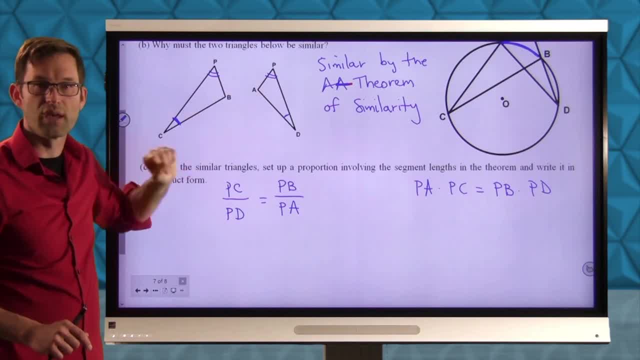 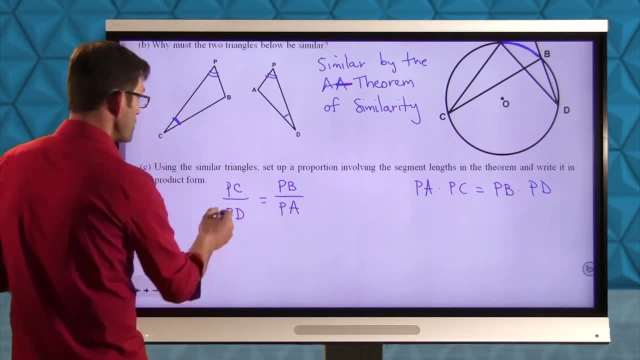 triangle is equal to short side of this triangle divided by short side of that triangle. PC divided by PD is equal to PB divided by PA. But now I can write it in product form And in fact I can just sort of cross multiply if you will, and I get exactly what I want. 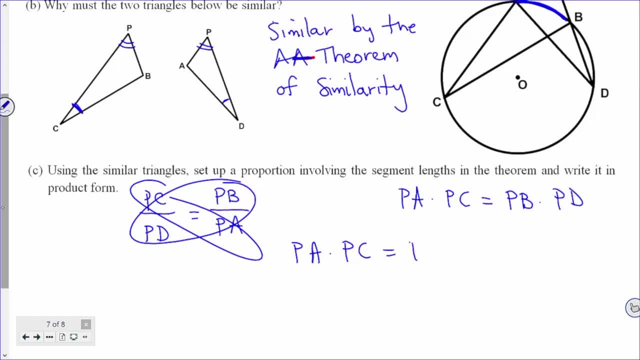 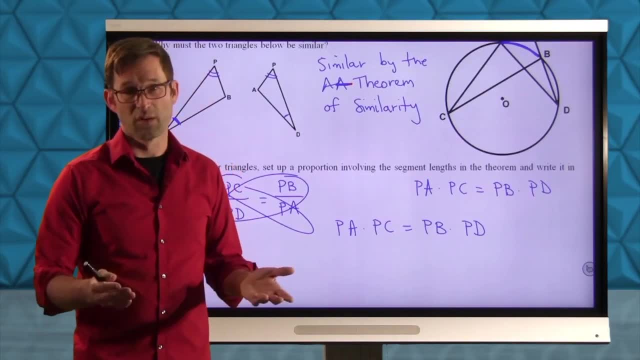 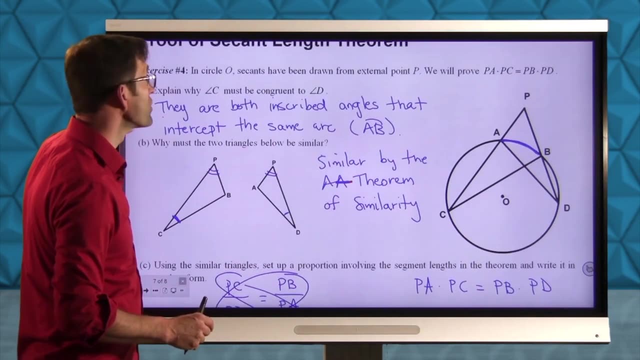 PA times PC is equal to PB times PD, And the reason for that would be: the product of the means is equal to the product of the extremes. So it's really kind of cool. This theorem that we were using today is a result of similar triangles. That similarity. 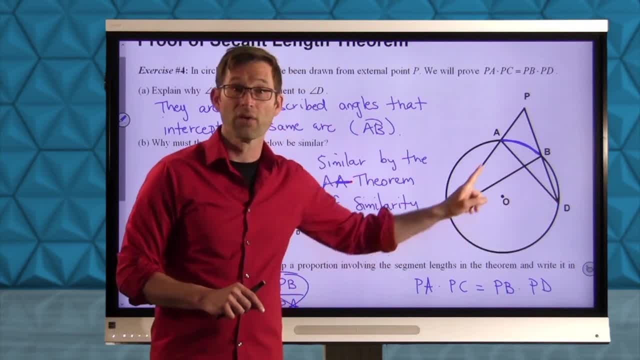 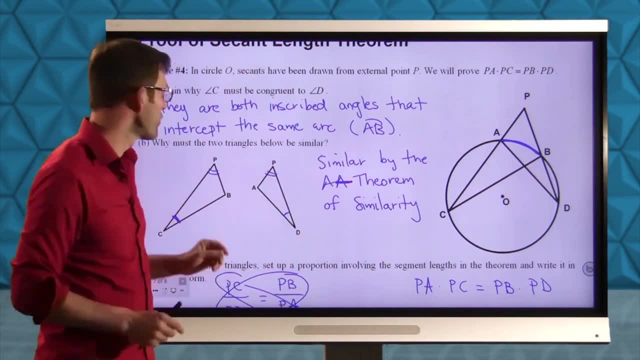 being caused by the fact that two angles, two inscribed angles that intercept the same arc, must have equal measures. Isn't that great How math kind of brings it all together in the end. All right, Let me pause now so that you can write down anything you need to. 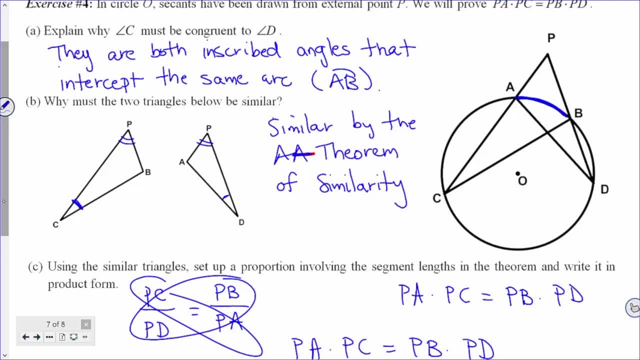 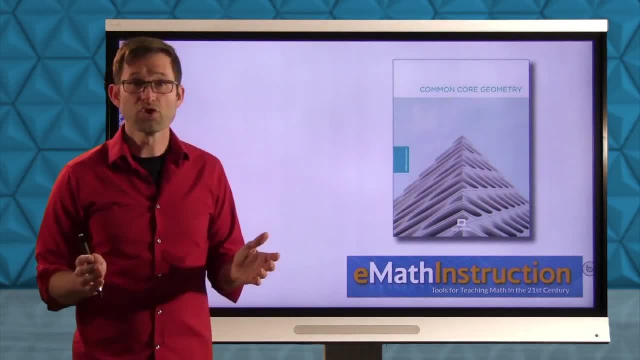 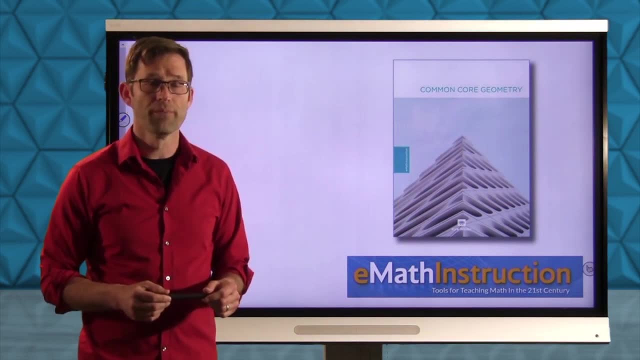 and then we'll wrap up. All right, Let's do it: Wrap this lesson up. So this lesson was a fairly short one, because it really presented a fairly simple theorem, Which is, if two secants intersect outside of a circle, then their segment lengths are. 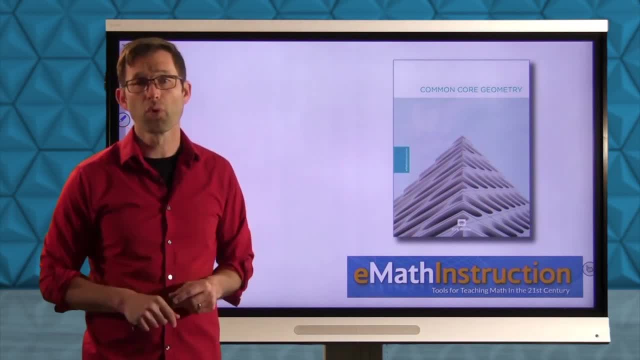 related by being able to take the product of the exterior portion of the secant times the entire length of the secant and that product remains constant, All right. So any circle if you locate a point outside of it and you draw two secants. 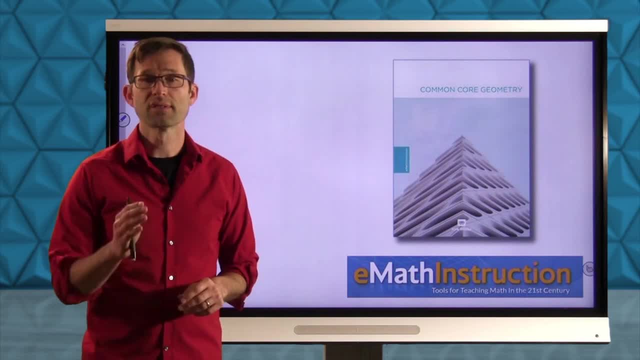 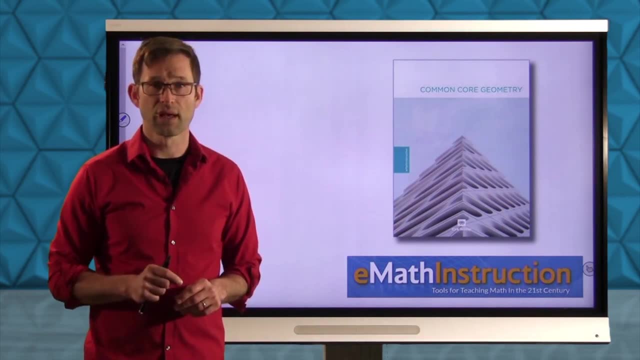 the products of those external segments with the entire segment stays constant. When it comes to a secant and a tangent, the product of the exterior portion of the secant is a tangent. since the entire portion of the tangent lies outside of the circle, it's.